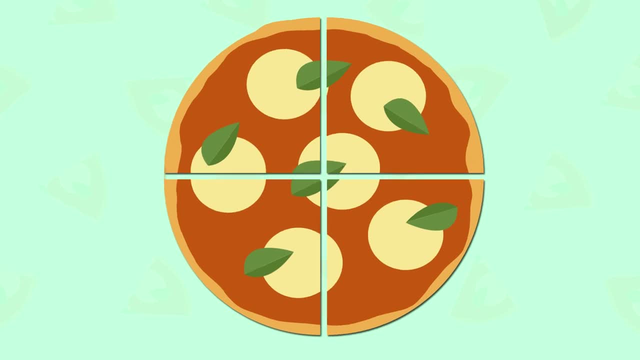 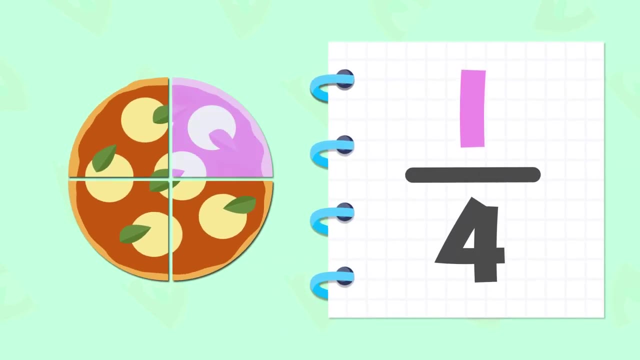 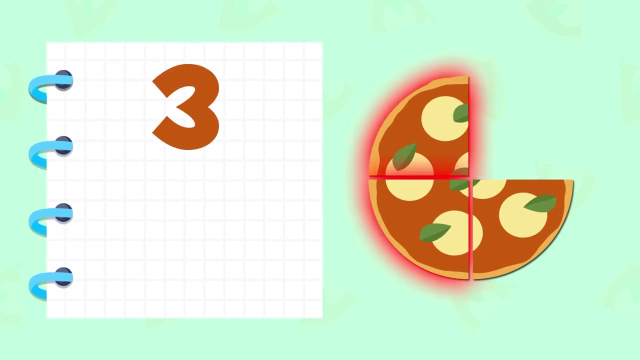 This pizza, for example, If we divided it in four equal parts and ate one of them, we would have eaten one-fourth of the pizza. The rest stays in the box. What fraction would that be? Well, if there are three alike pieces left in the box- and there were four pieces before- there are three-fourths of pizza left. 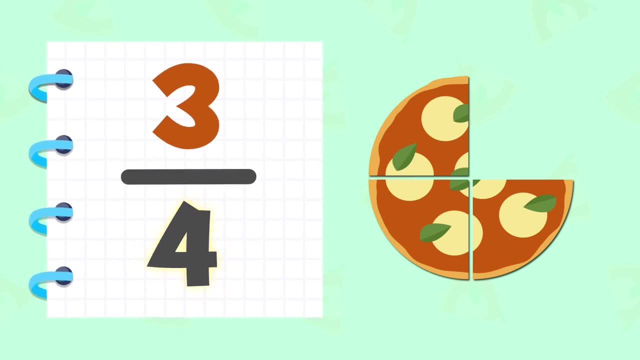 That's it. The number below the line is the denominator. It indicates into how many equal parts the object is divided. In this case it's divided in four parts. The numerator is the number above the line. It indicates the number of parts taken away from the whole. 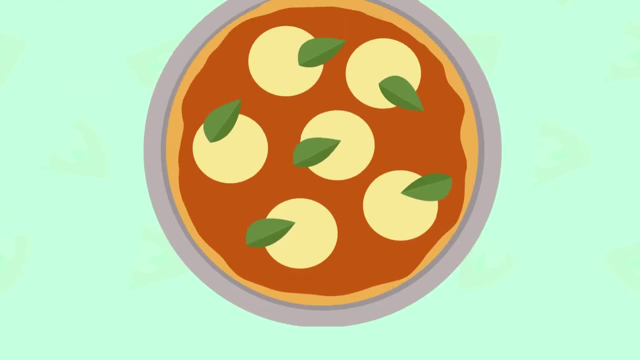 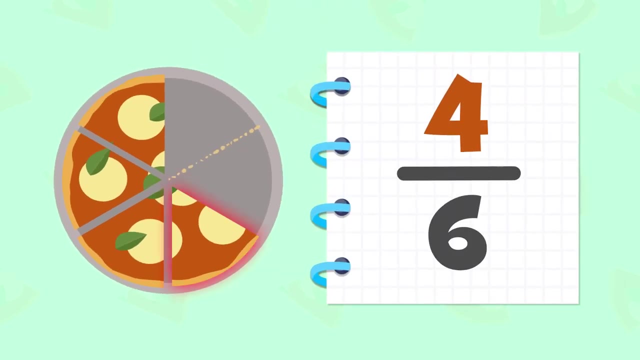 And if we divided this last pizza in six parts and ate two, there would be four-sixths of pizza left in the box. How many have we eaten? Two-sixths. Very well, Mario, You've earned yourself a swell dessert. But before that shall we recap. 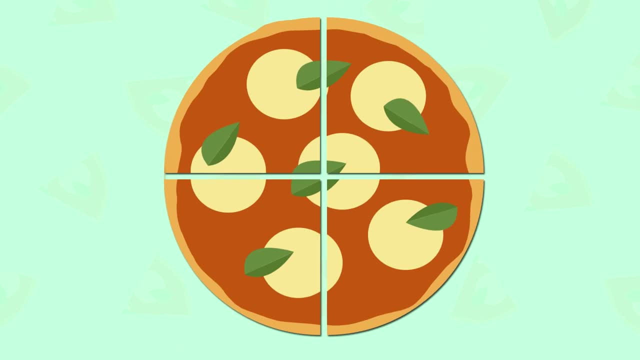 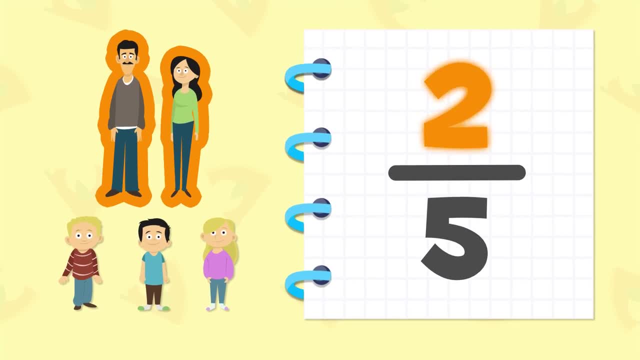 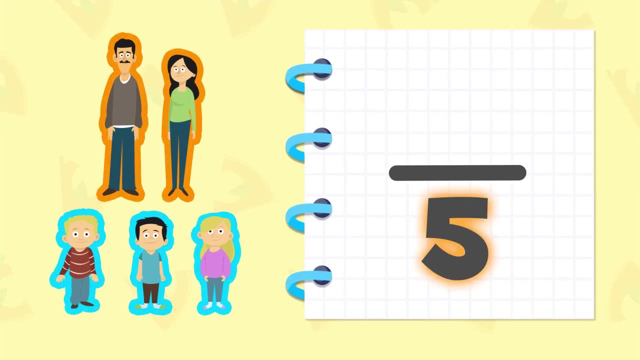 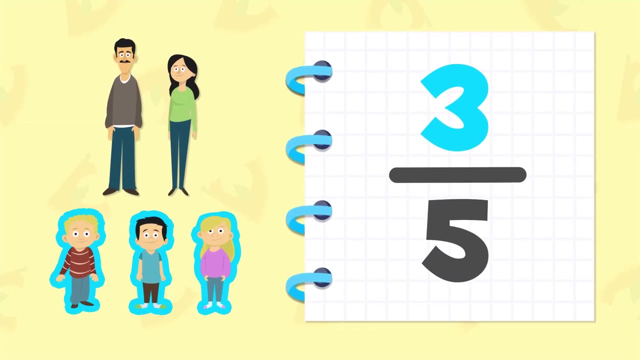 And the numerator represents the elements we have selected, And the numerator represents the elements we have selected. We are five in this family. We are five in this family. Three of us are kids, Three of us are kids, So three-fifths of our family are kids. 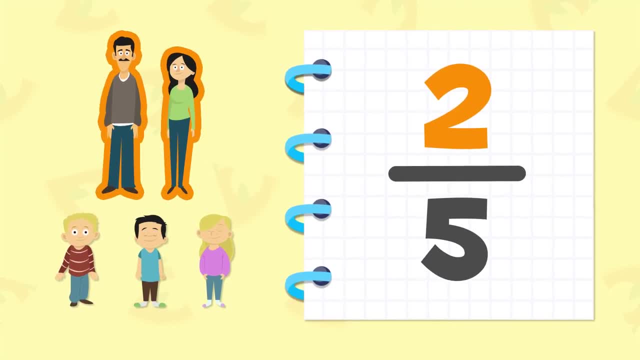 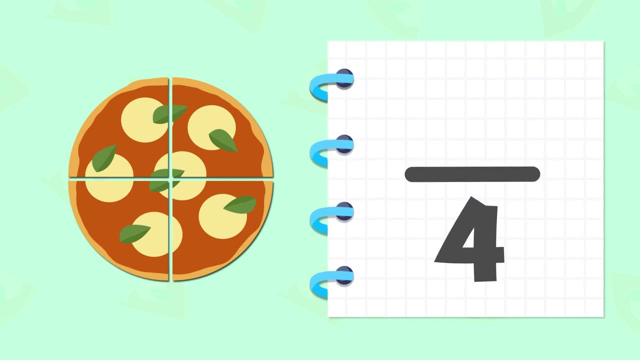 And two-fifths of the group are adults, That's mom and dad. We could also see fractions when we divided an object into equal parts. The denominator represents the number of parts in which the object is divided And the numerator represents the part of the fraction we are talking about.